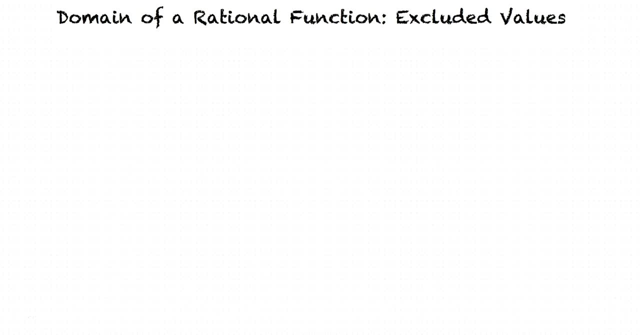 This video will cover the topic Domain of a Rational Function- Excluded Values. What do you mean by the domain of a function? By definition, domain of a function is the set of all inputs for which the function exists. On the other hand, excluded values are values for which the function does not exist. 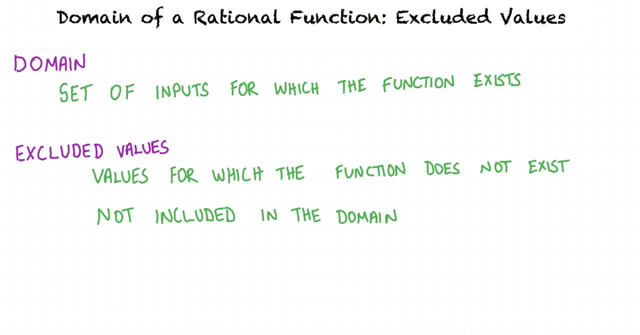 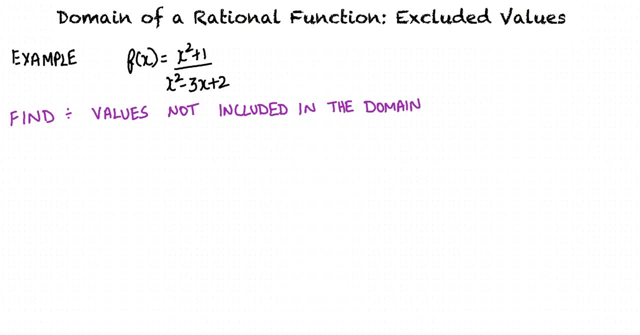 and hence excluded values are not included in the domain. Let us consider an example. Let's say we have a function f of x equals x square plus 1 over x square minus 3x plus 2, and say we are required to find the values that are not included in the domain of the function f of x. 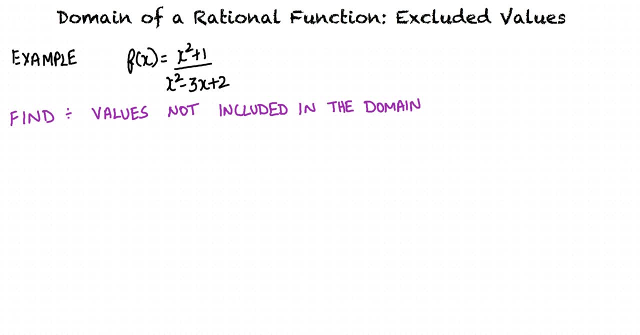 In other words, we are asked to find the excluded values in the domain of the function f of x. By definition, excluded values are the values for which the function will not exist. Under what circumstances will the function not exist in this case? The function will not exist when the denominator becomes 0, right. 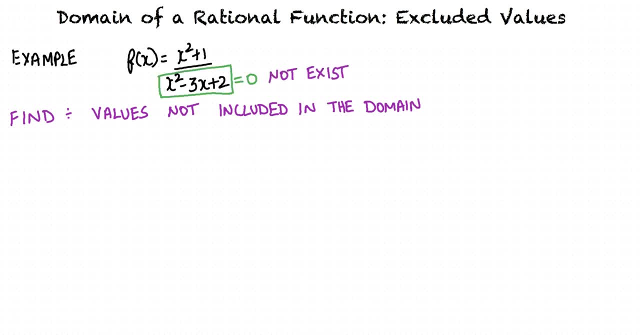 Correct. The function will not exist when the quadratic expression in the denominator equals 0. Thus, to find the excluded values, we equate the denominator to 0 and solve the equation for x. We get x square minus 3x plus 2 equals 0.. 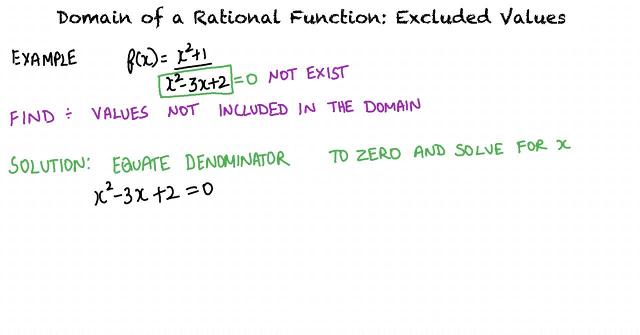 Determining the factors of the quadratic expression and equating it to 0,, we get x equals 2 and x equals 1.. When x equals 2 and x equals 1, the function ceases to exist, and hence 2 and 1 are the excluded values of the function not included in the domain. 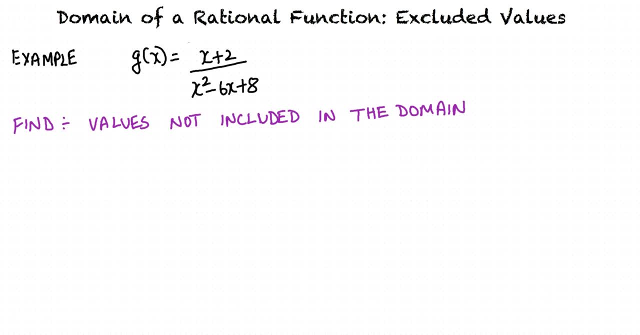 Let us consider another example. Let's say we have a function g of x equals x plus 2 over x square minus 6x plus 8.. Say we are required to find the values not included in the domain of the function g of x.